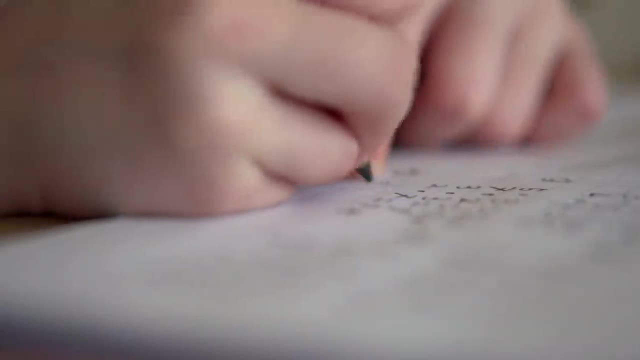 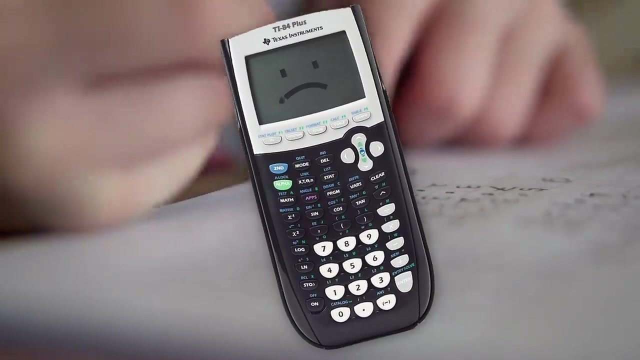 This is because it's the problem at the core of problem solving itself. So, yeah, you can put away your TI-84,. you're not going to get a million dollars by typing a bunch of numbers into a wildly overpriced paperweight from 2004.. This is fancy math. 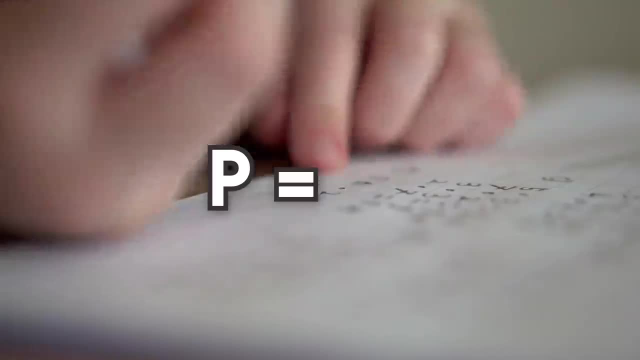 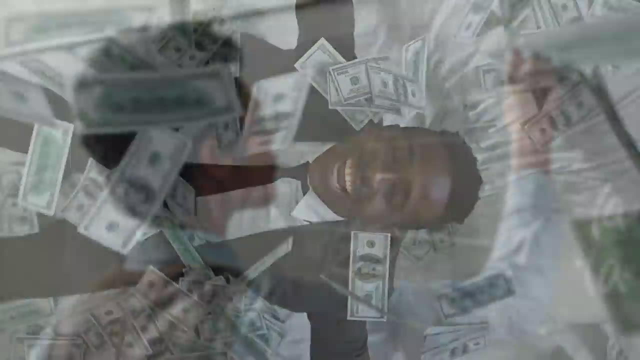 Technically, this problem asks the question: does P equal NP? And before you say no one of them has an N stuck to it, gimme the prize money. what this question really means is: can a problem with an easily verifiable answer also be easily solved If it turns out that 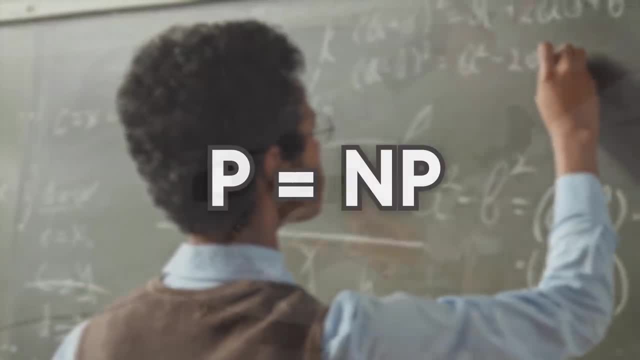 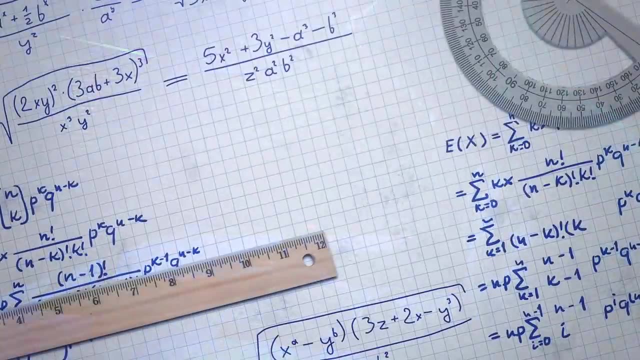 it can and P does equal NP. we would be able to use the proof to literally cure cancer and hack Jeff Bezos' bank account at the same time. We'll get to that bit later. First, I should explain what P and NP stand for here. P represents all of the problems. 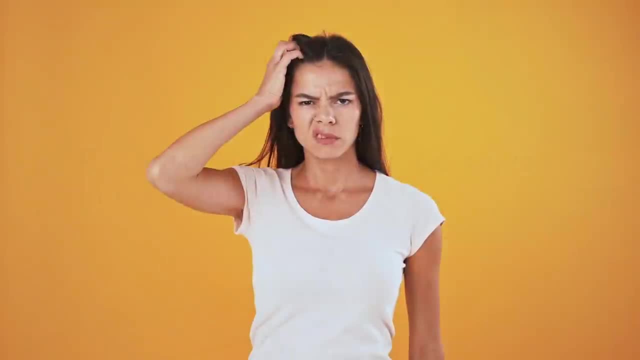 that can be solved in polynomial time or in words that can be understood by normal people who don't already know all of this and aren't just watching this video to point out all the mistakes I'm about to make. it represents all of the problems that can. 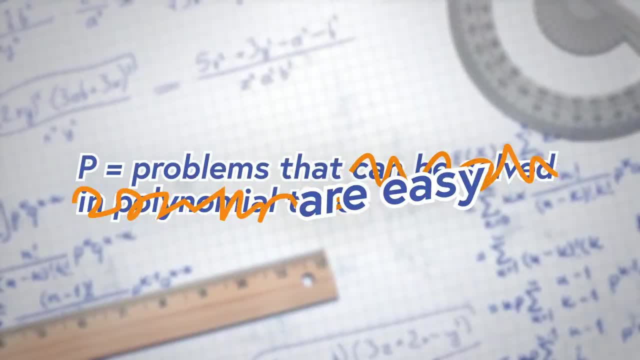 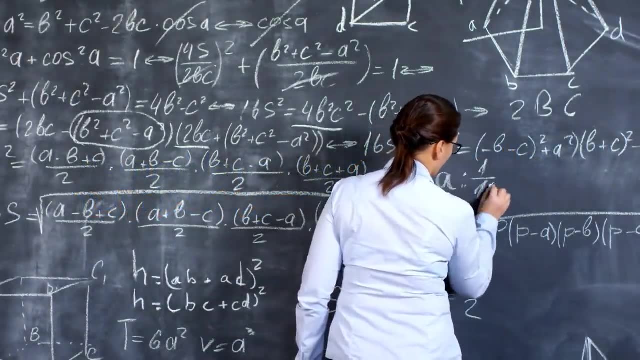 be solved with an algorithm in an amount of time that doesn't get exponentially longer the bigger they get. Most basic math problems fall under this category, like, for example, calculating a tip, Whether you're dealing with a three dollar muffin or a three million. 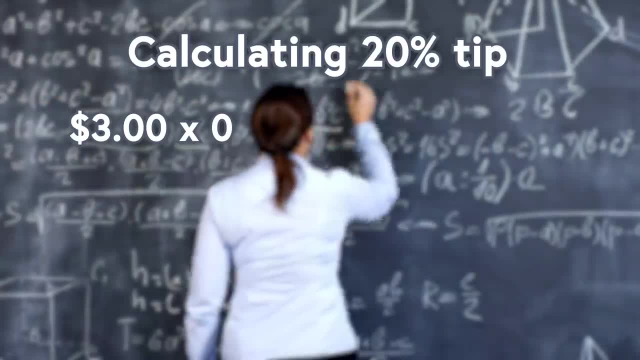 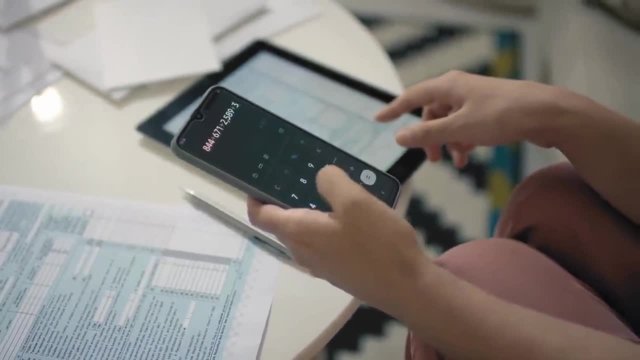 dollar muffin that you're using for some very convoluted money laundering scheme. calculating 20% is pretty much the same process and your phone could calculate a tip on any muffin, no matter how much money you're laundering- pretty much instantaneously. 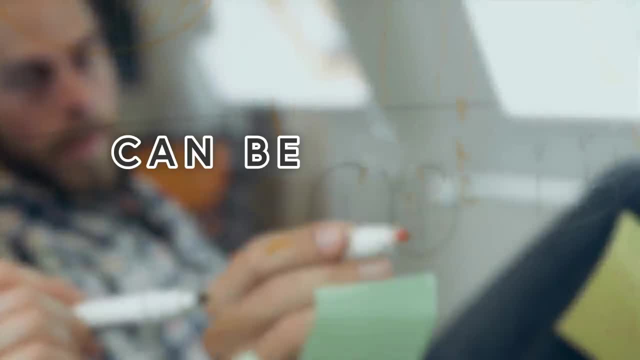 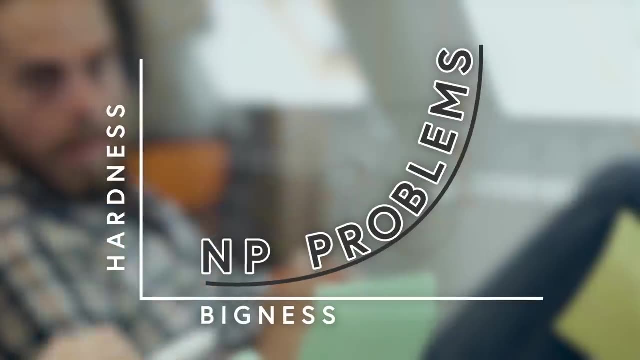 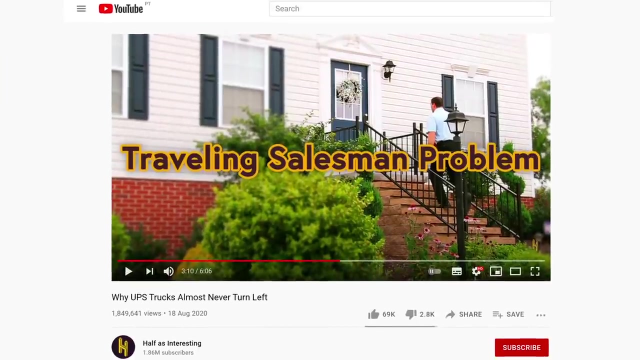 NP problems, however, are different. While they can be checked in polynomial time, they can't necessarily be solved in polynomial time—that just means that solving them gets exponentially harder the bigger they get. Take, for example, the traveling salesman problem. You might remember that we talked about it in this video, where we explained. 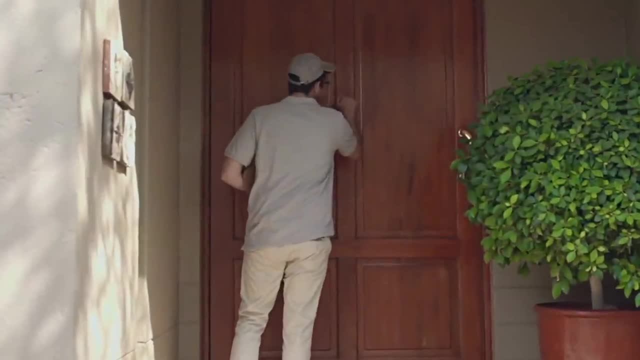 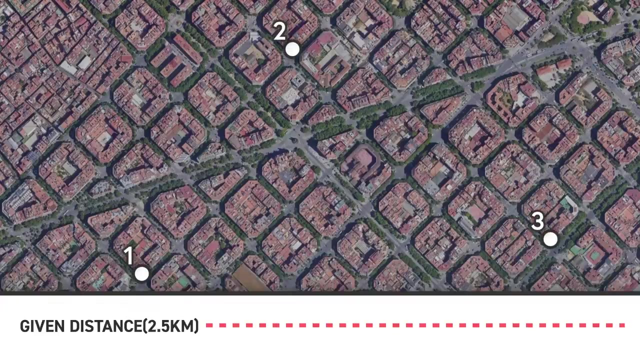 how it's the postal service's biggest obstacle to getting you your week-late Father's Day present 15 minutes faster. The problem works like this: Given a handful of destinations and a certain distance, is there any way to tell if there's a route between all of the 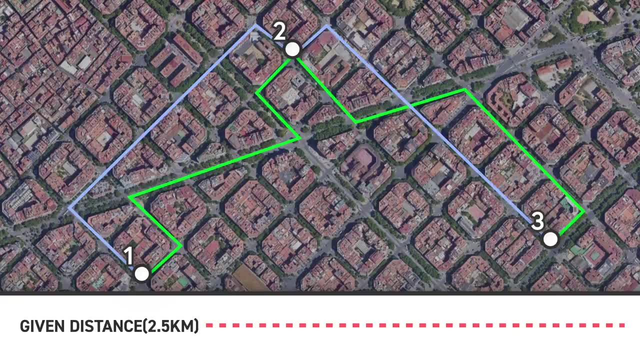 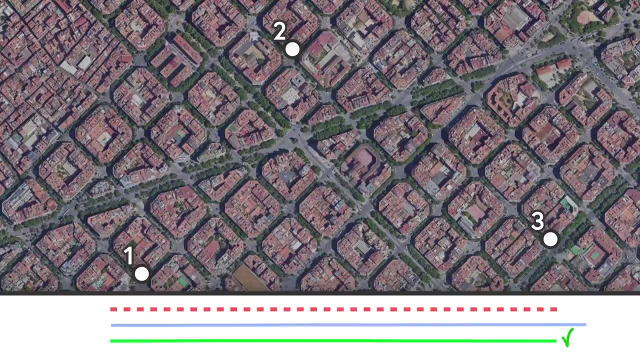 destinations that's shorter than that distance. Well, it's easy to check any given answer, since you can just measure the length of the route. but there's actually no efficient way to find the correct answer. You just have to try every possibility until something works. 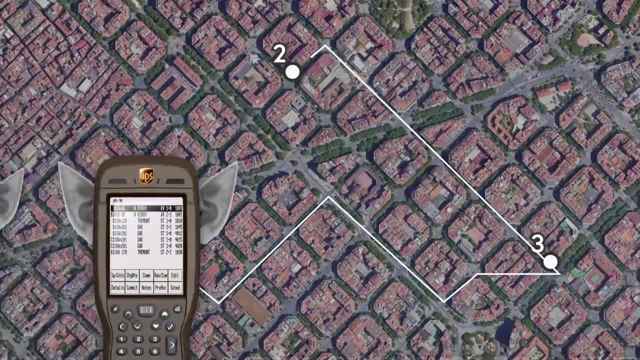 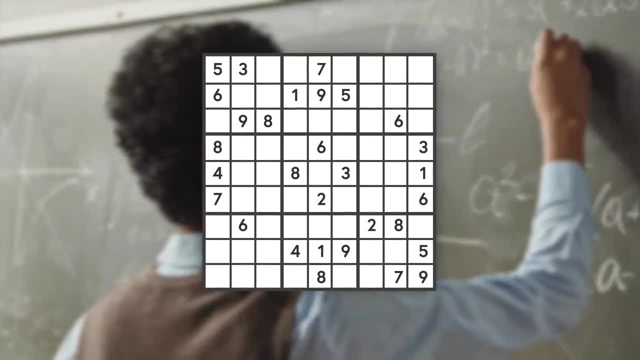 which can take a really long time and take a lot of time. So let's just say that you're trying to find a route that's shorter than that distance. Another example of an NP problem would be Sudoku. There's no algorithm for efficiently solving. 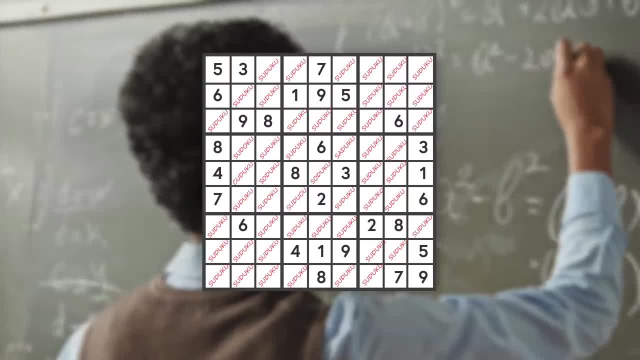 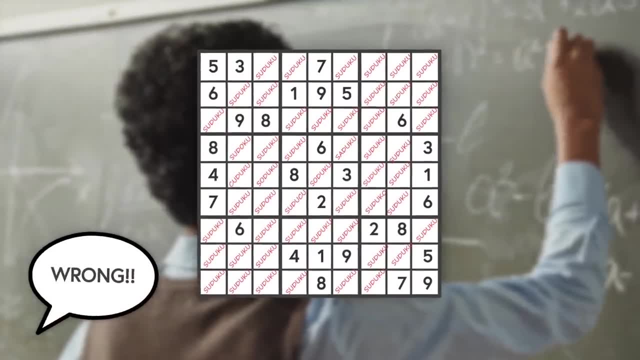 a Sudoku. but if I gave you a Sudoku that I had already filled out, you could pretty quickly check to see if it was right and then after about two seconds you could tell me that it was wrong, because I had just written Sudoku into the boxes over and over again. and I didn't even spell it right most of the time. There are some problems that we thought belonged to this category of easily checked but not easily solved, like determining whether it's prime or not- but then we found an algorithm for solving them, and they. 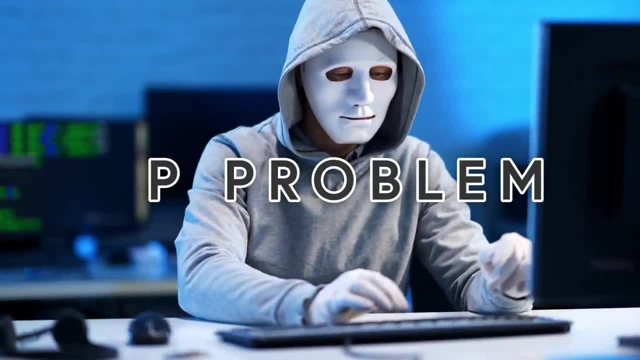 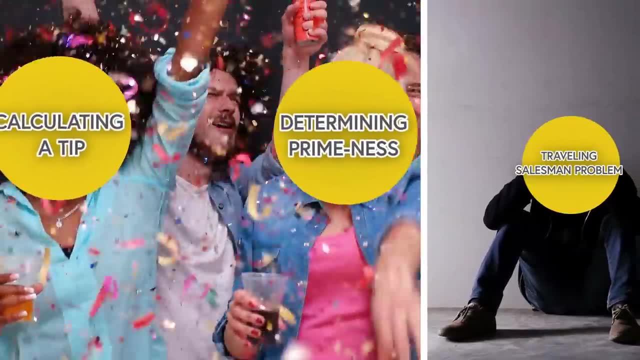 ascended to p-status. So the question is: is there something about these other problems that makes it impossible for them to join their friends in the p-party, or are they all theoretically solvable, Or in other words, are all checkable problems eventually going? 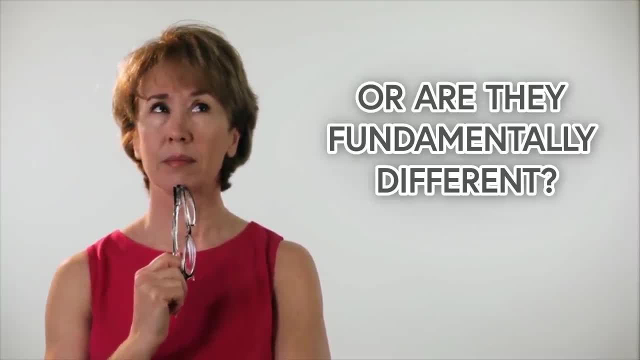 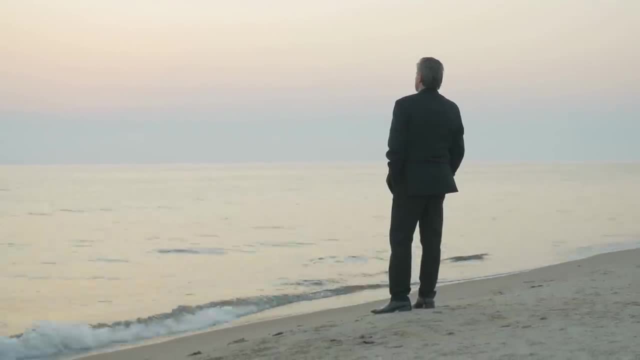 to be solvable problems, or are they fundamentally different in some way? Well, when you're dealing with an infinite number of problems, that seems like an unanswerable question. but it turns out to be a very simple problem, and that's what we're trying. 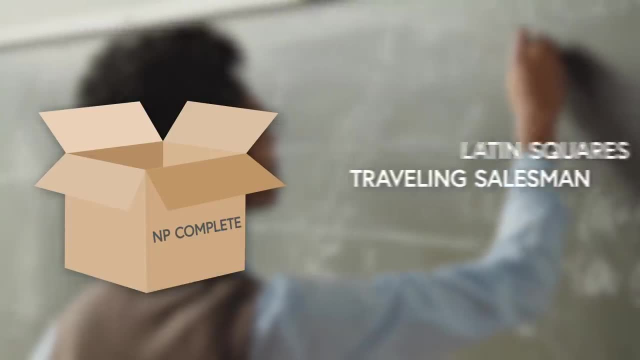 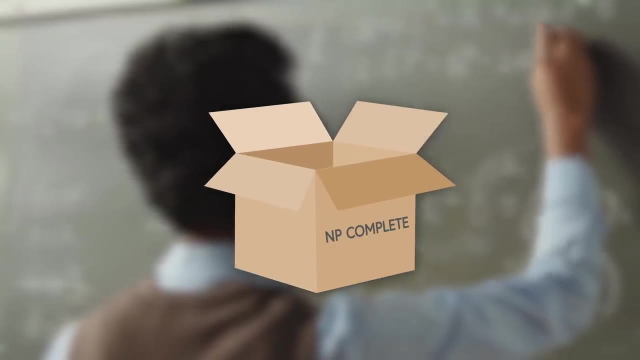 to solve. But it turns out that a bunch of these problems, like the traveling salesman problem and Sudoku, are actually technically the same problem at their core, and this problem happens to capture the most difficult aspect of NP. This means that if you come up for 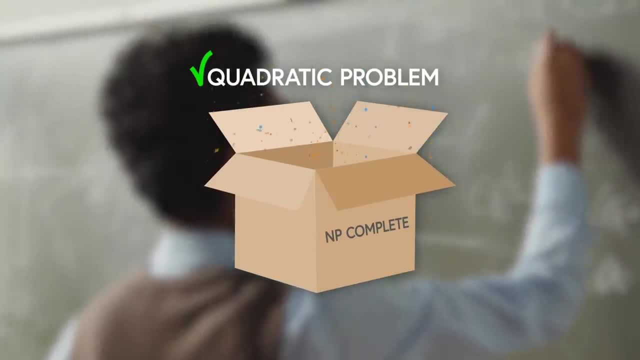 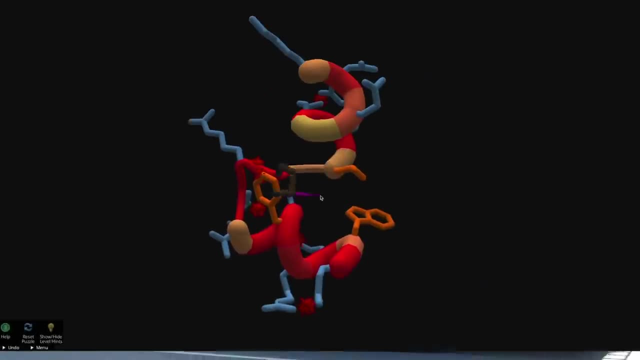 a proof for one of these so-called NP-complete problems. you can use it to solve everything else in NP. You could use it to route packages with 100% efficiency or accelerate our methods for protein folding, But you would also break most of our current financial encryption systems. 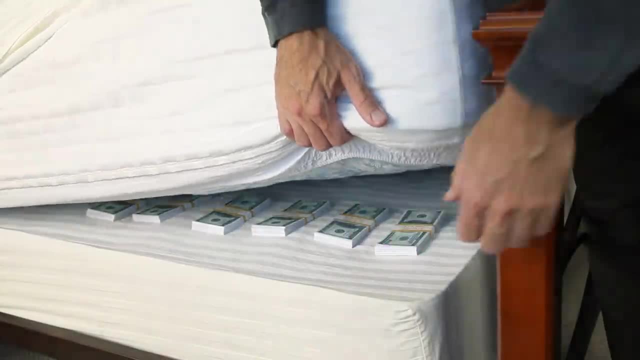 so you'd probably have to hide that prize money under your mattress. So I was going to tell you that once you won a million dollars from solving one of these problems, that you should invest in a quality kitchen knife. but it turns out you. 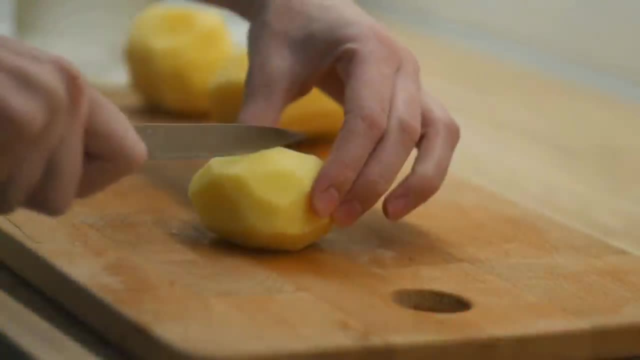 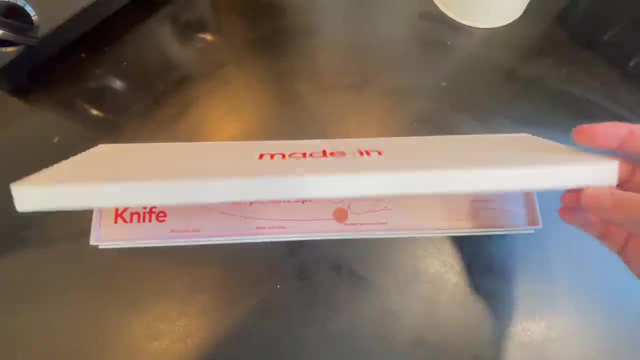 don't need a million for that. My least favorite part of cooking used to be the prep—dicing potatoes, mincing garlic, trimming meat- you know the knifey bits. But then I got this—the chef's knife- from our sponsor Made In. I sliced some cantaloupe, tried to catch my 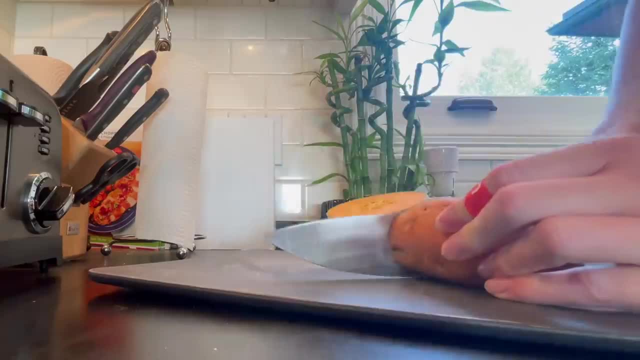 phone with the hand, with the knife, found out why the box includes a mandate. sliced some sweet potato and, man, was that the most pleasurable sweet potato slicing experience I've ever had in my entire life? So here's what you need to do to solve these problems.